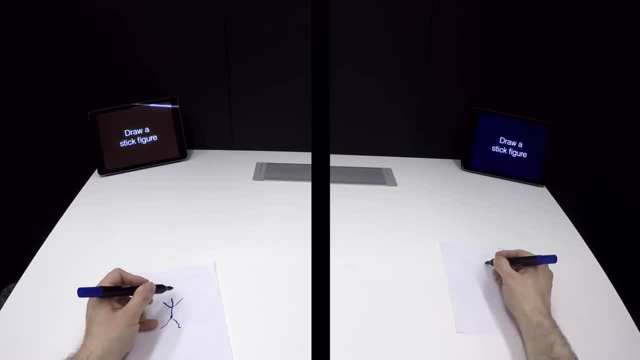 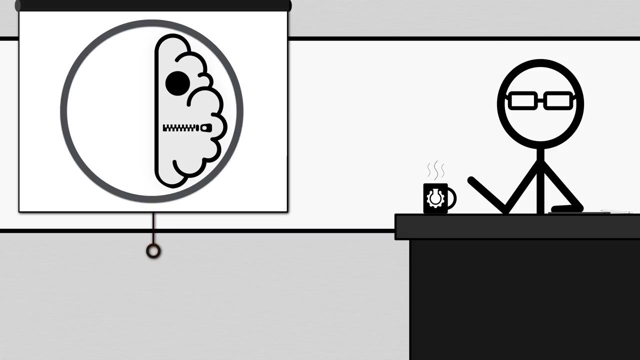 I'm not holding anything And when asked to draw, a split brain can draw two separate objects simultaneously with each hand. in a way, unsplit brains find challenging. These experiments on split brain patients are deeply unsettling because they really point in the direction of a mute, separate intelligence, something living in the skull. You can even ask: 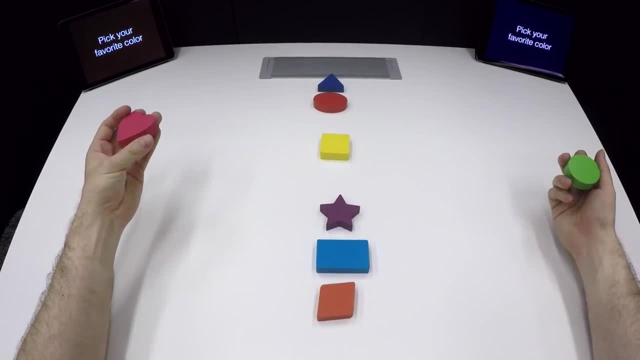 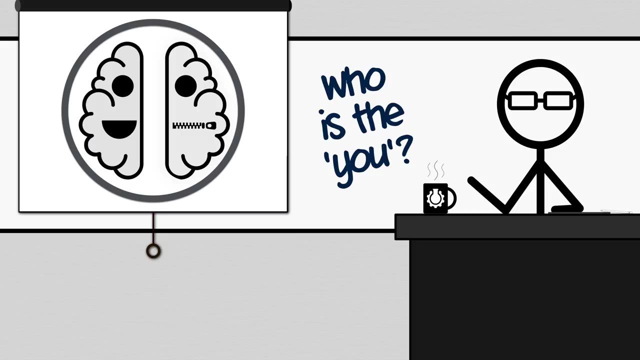 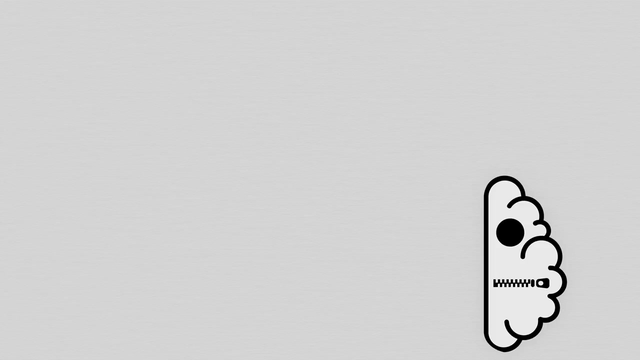 questions of a split brain and get disagreement on the answer. So if your brain is split, who is the you in this situation? From the outside it's tempting to think of the part of the brain as the person, but something is hearing and answering questions, And though right brain. 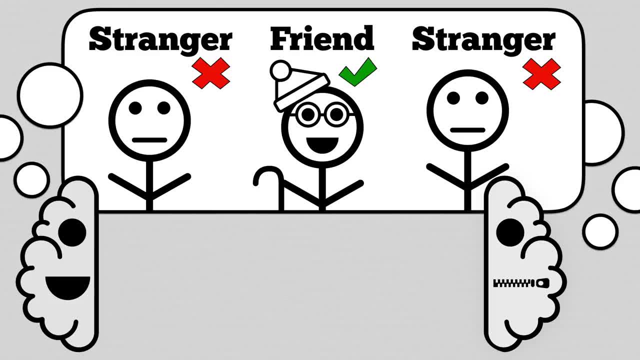 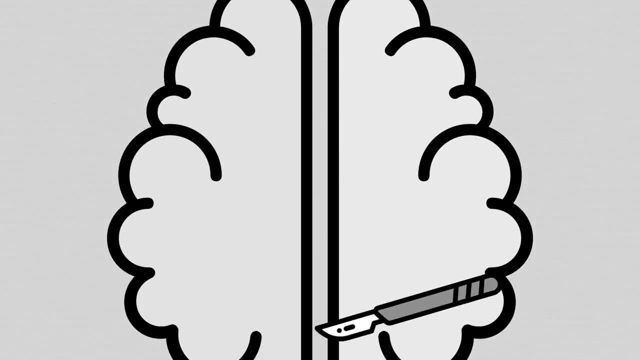 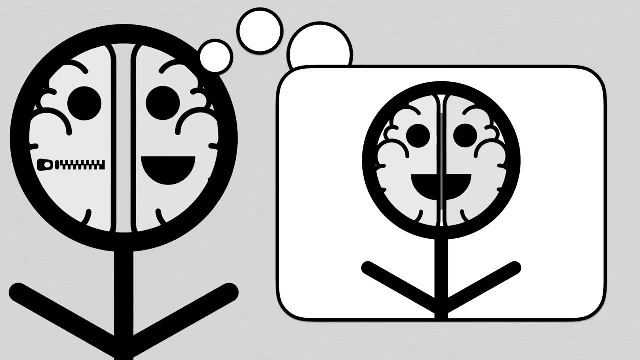 can't speak, it does understand faces, which left brain can't. If this is you, you don't know who your friends and family are in a crowd. This act of cutting exposes two minds in one head, and the talking mind doesn't know there's someone else in the house. The left brain can describe the. 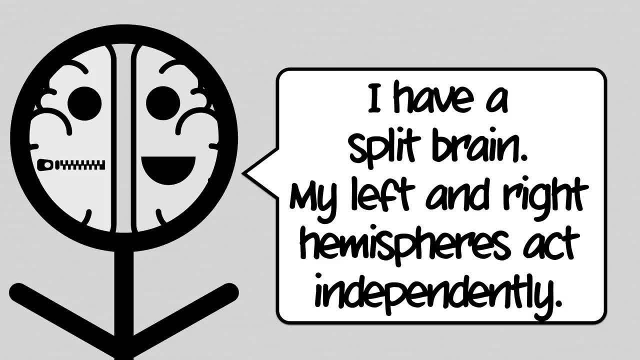 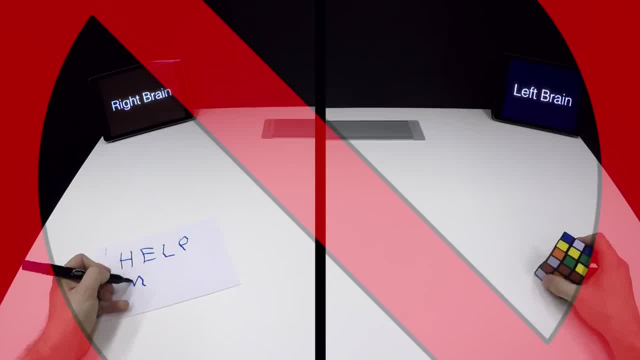 situation it's in but nonetheless will constantly be surprised by right brain's actions and explain them away. There's a question to be asked here: Why, after separation, does right brain not totally freak out but instead plays along helpfully answering questions? 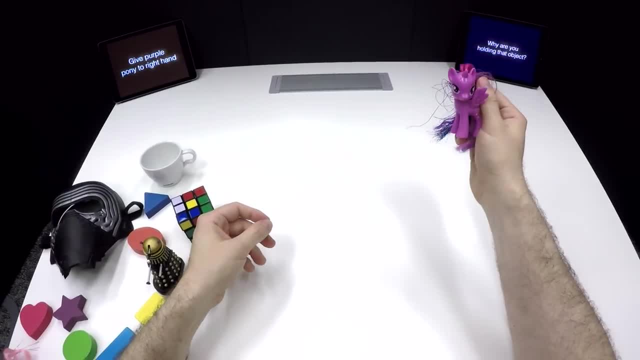 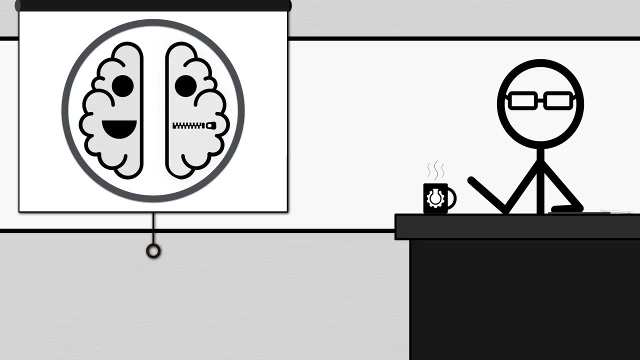 and listening to left brain's dumb stories about what's happening. It's the best pony, I don't know, Speculation time, But one answer is: the cutting doesn't make right brain a separate intelligence consciousness person, but rather it has always been In normal people. perhaps right brain grows up to be the most intelligent person in the world, but in left brain it's the most intelligent person in the world. Perhaps right brain grows up to be the most intelligent person in the world. Perhaps right brain grows up to be the most intelligent person in the world. Perhaps. 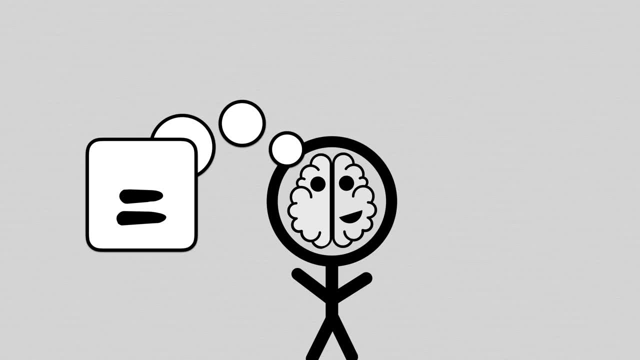 left brain grows up to be the most intelligent person in the world. Perhaps right brain grows up as a companion without a choice, feeling at first somewhat equal partners, but then, as speech develops that it can't participate in, that increasingly becomes the central point of life. 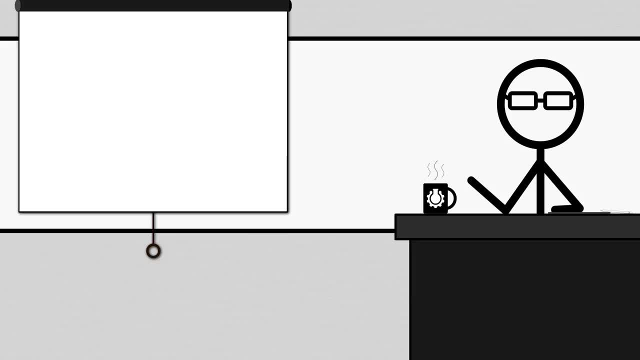 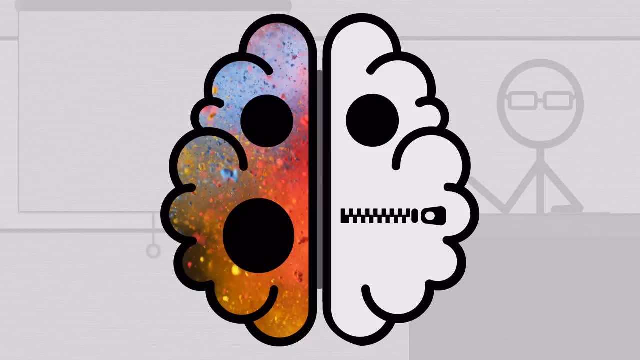 it resigns to mutely coordinate with left brain. At this moment, in your normal head, there are two of you watching this video, One having a mind equals blown moment and the other mentally rolling its eye at the obviousness of it all.